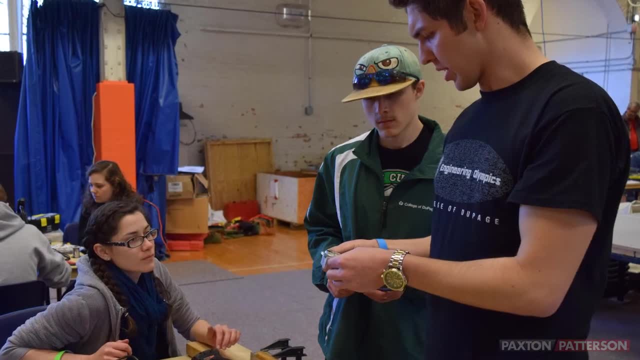 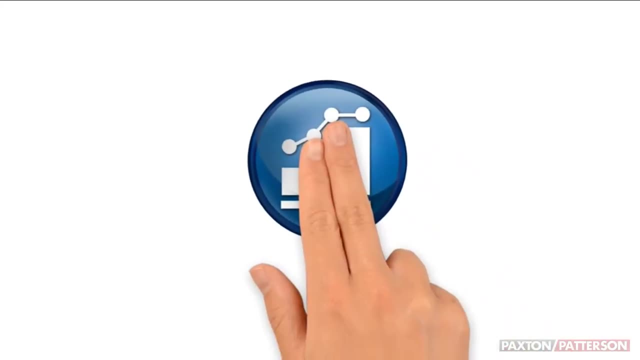 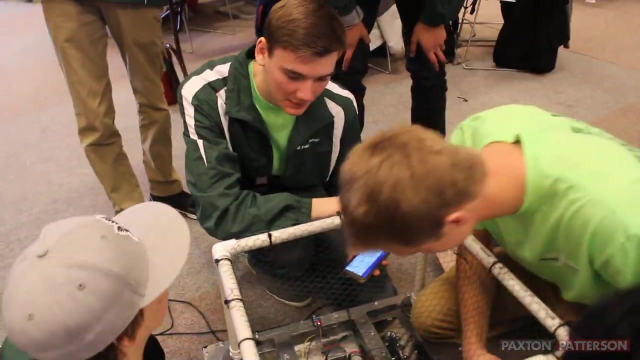 something great that could lead to a possible solution. Designers should document all the ideas generated in their engineering design notebook. Stage 3 – Evaluate By this stage in the engineering design process there should be multiple potential solutions to the problem. The engineers compare ideas. 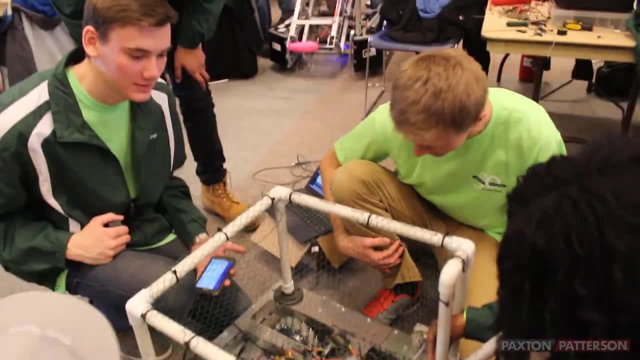 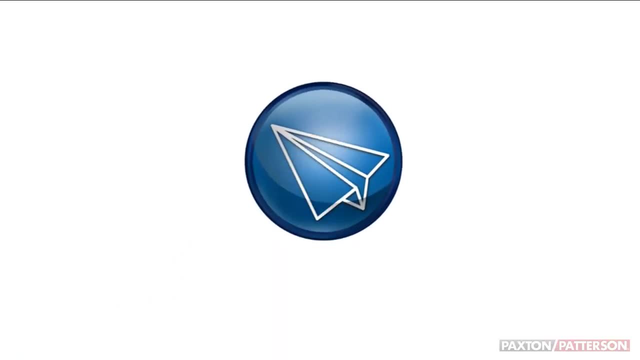 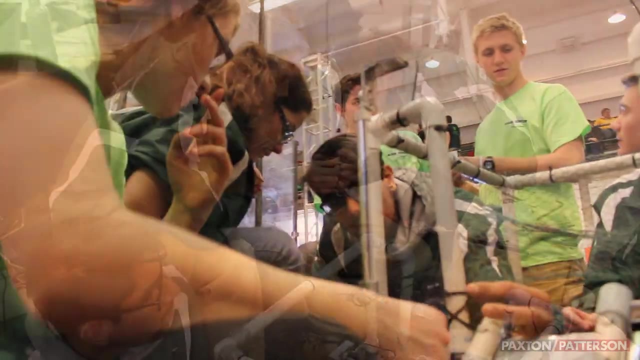 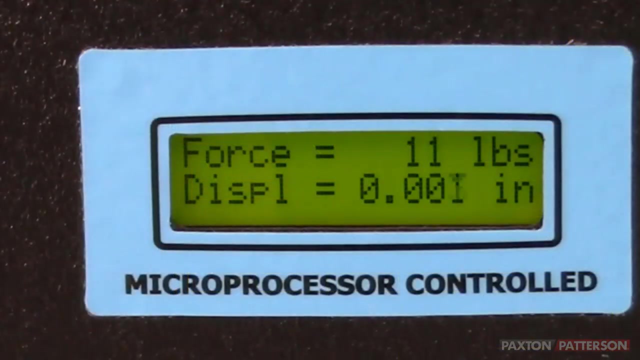 and evaluate how each one fulfills the specifications. They then determine which solution is best. Stage 4 – Create. Engineers take the agreed upon solution and create models or prototypes. These may be constructed as full-scale models or small-sized versions. Diagrams or graphs can be used to help visualize the basic functions or features. along with computer and mathematical models. The goal is that the students can visualize the basic functions or features, along with the computer and mathematical models. The goal is that the students can visualize the. The goal is that the students can visualize the basic functions or features, along with. 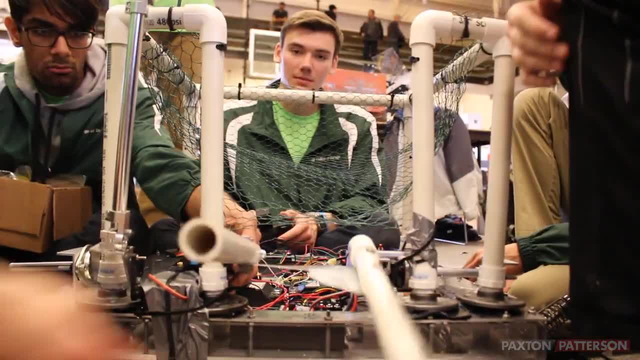 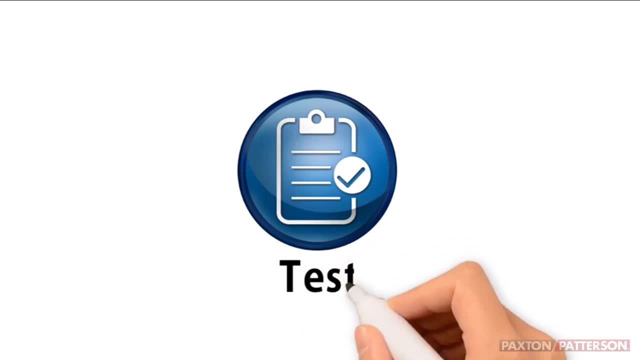 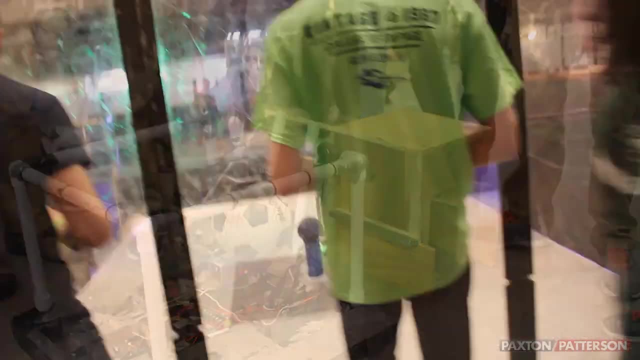 The goal of this stage is to learn how the solution will function in real life and how it interacts with the real environment. Step 5 – Test and Refine. In the final stage of the engineering design process, engineers will perform a variety of tests to evaluate the design solutions and compare it with the goals. 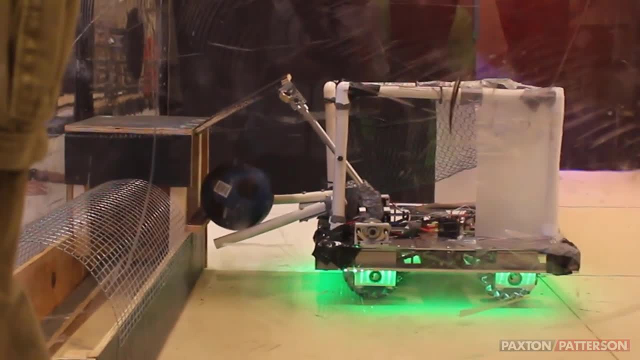 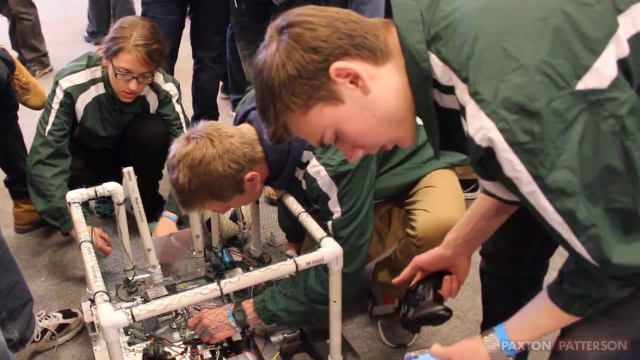 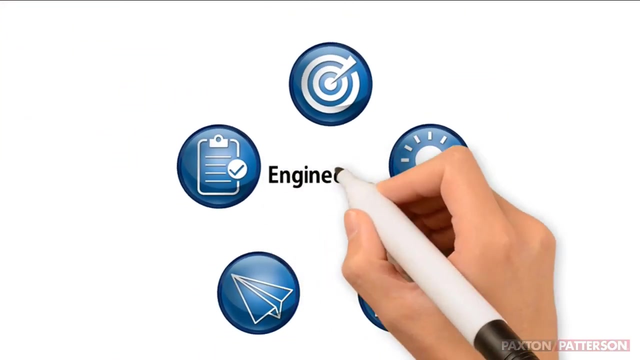 They can then decide whether to proceed with the design solution or to start all over again. If approved, the design solution may be refined if needed before proceeding to the manufacturing and construction stage. And those are the five basic steps of the engineering design process – Define, Imagine, Evaluate, Create and Test. 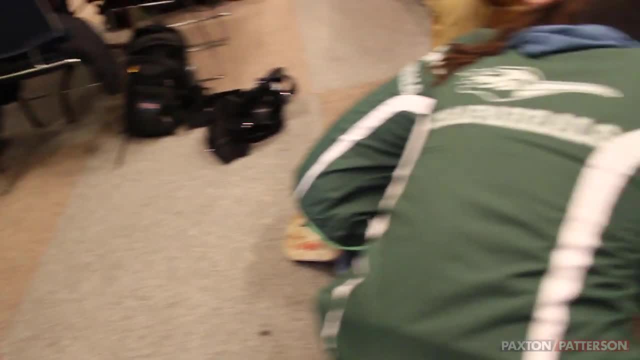 It's important to note that the designers typically develop multiple versions of a design before calling it final, and the engineering design process is not always linear. It's important to note that the designers typically develop multiple versions of a design before calling it final, and the engineering design process is not always linear. 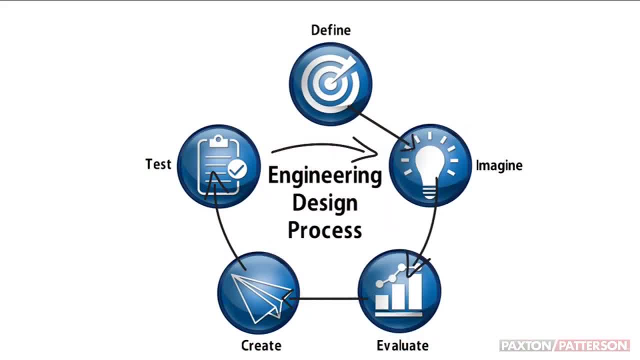 It's important to note that the designers typically develop multiple versions of a design before calling it final, and the engineering design process is not always linear. It is common to jump from stage to stage and revisit stages several times before moving on. The longer the design process goes on, the more problems will be discovered and improvements made.